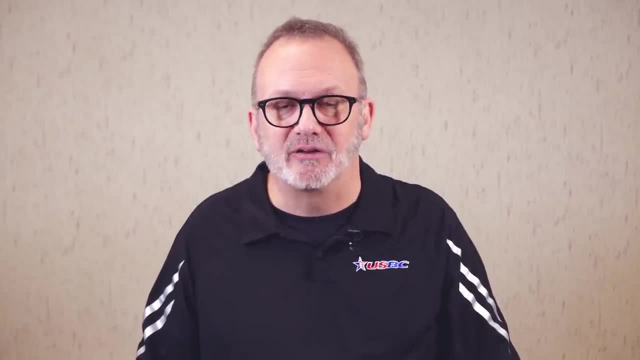 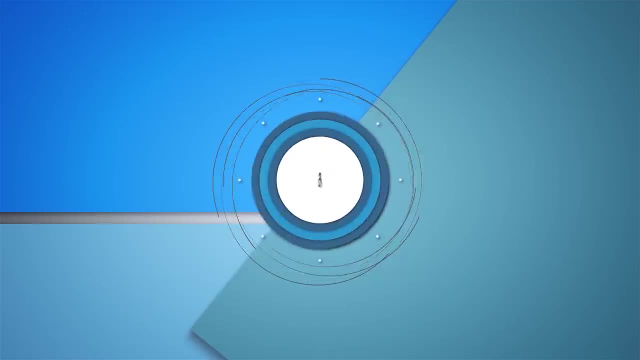 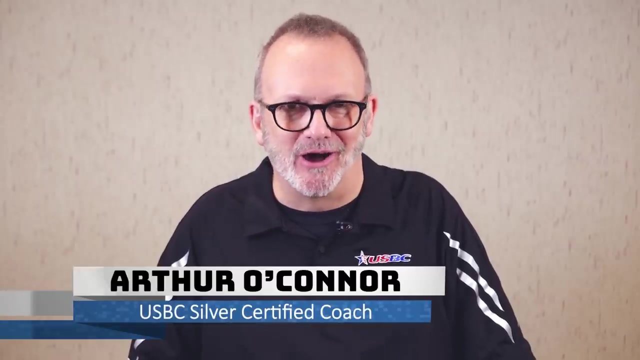 We're going to look at some of the physics behind bowling and let you decide for yourself if 16 pounds is king of the lanes Coming up on The Art of Bowling. Hi, I'm USBC Silver Certified Coach Arthur O'Connor, Here at The Art of Bowling channel. 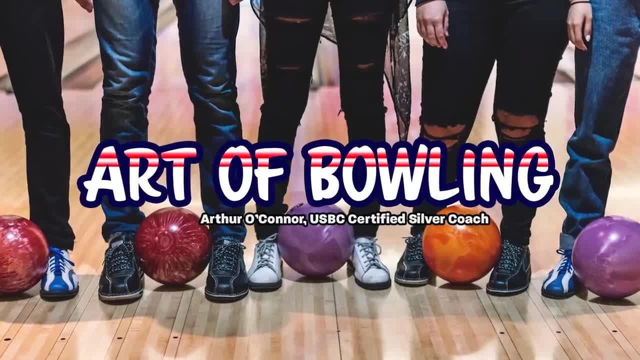 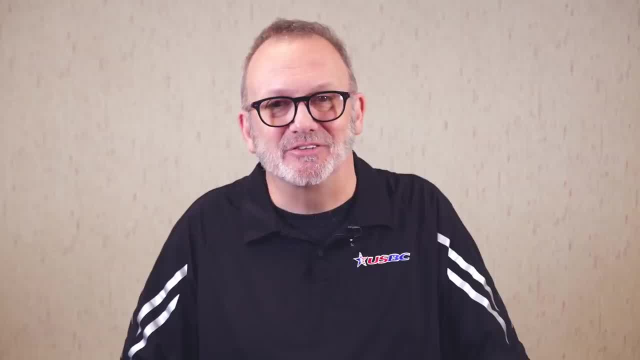 we discuss tips, tricks and techniques to help you bowl your best. If you haven't already, subscribe to our YouTube channel and hit the bell so you don't miss our next video. So how can 16 pounds not be the hardest hitting ball in the alley? Can a 14 or a 15-pound ball? 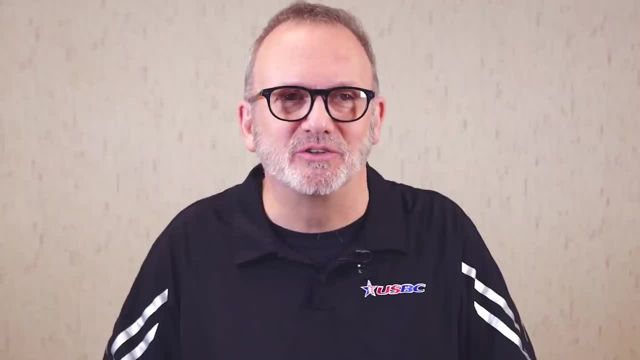 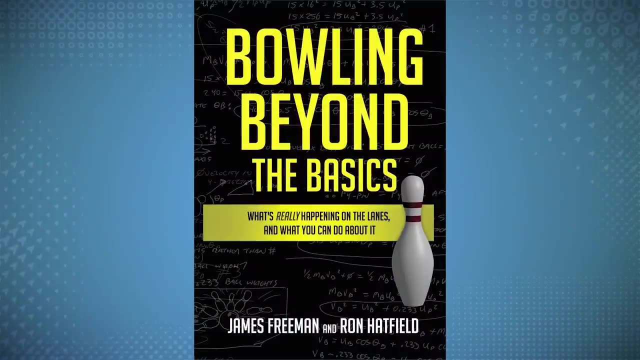 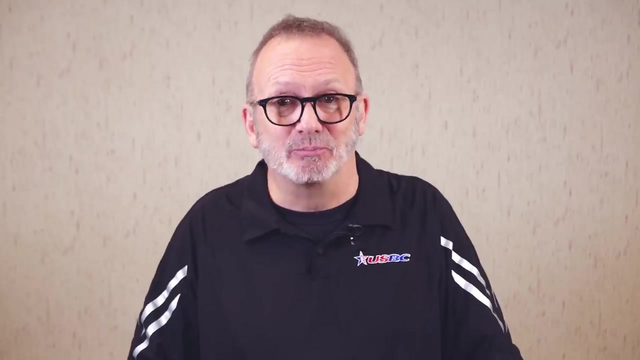 really hit the pins harder than a 16-pound ball. Before you dismiss this notion as mere poppycock, let's analyze this issue. In Ron Hatfield's book Bowling Beyond the Basics, he states that a 14-pound ball will in fact hit harder than a 15-pound ball. How can he? 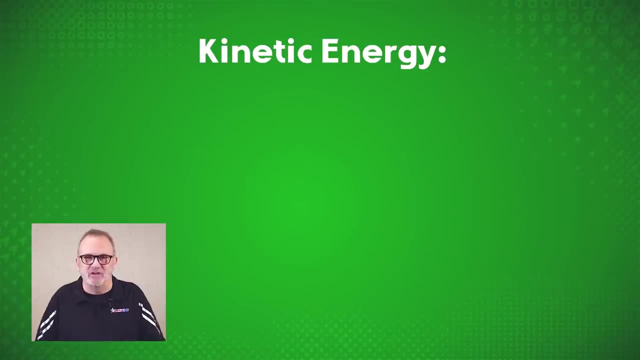 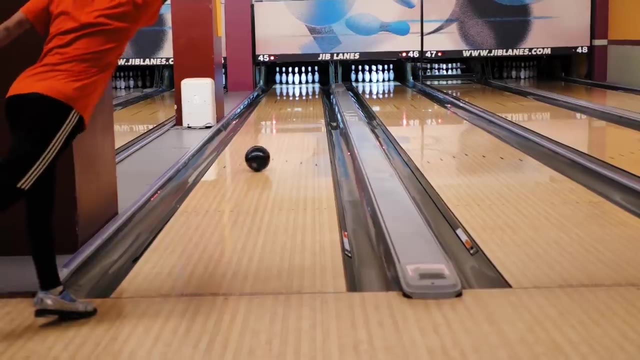 prove that statement with physics. Kinetic energy is the amount of energy that an object has due to its motion. The more kinetic energy in your bowling ball as it meets the pins, the harder it hits. Do you know the formula for kinetic energy? 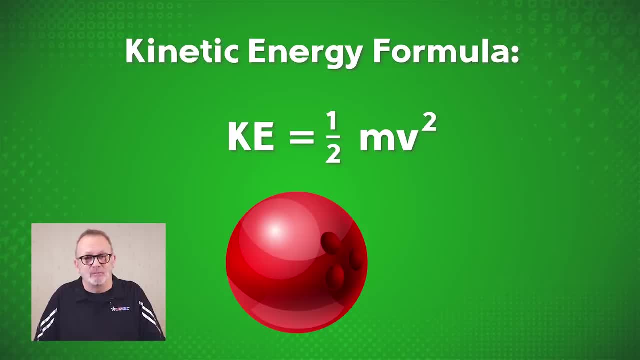 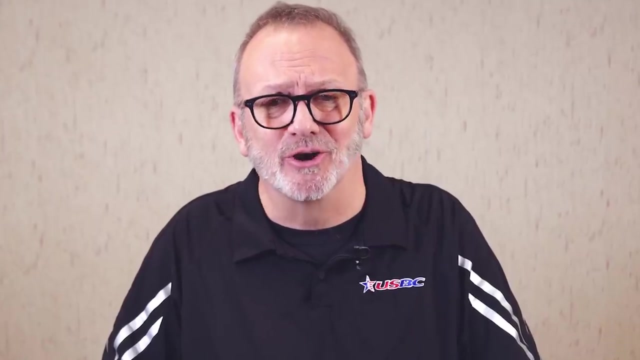 Yeah, One half mass times velocity squared. The formula for calculating kinetic energy in an object in motion is one half of its mass multiplied by its squared velocity, And the answer to this question is that kinetic energy is measured in a unit called joules. What does that mean for 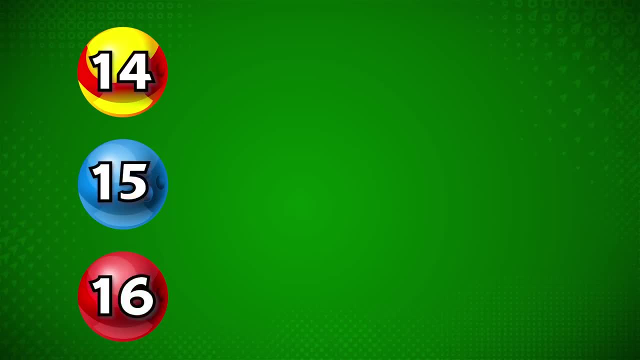 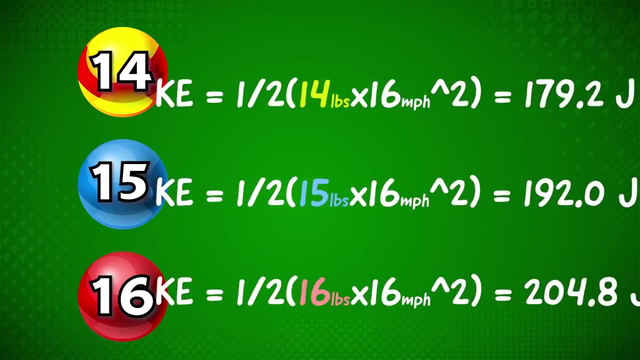 us bowlers. Let's look at this formula laid out for three different ball weights: 14,, 15, and 16 pounds. assuming speed or velocity stays the same, Let's say we throw the ball at 16 miles per hour. 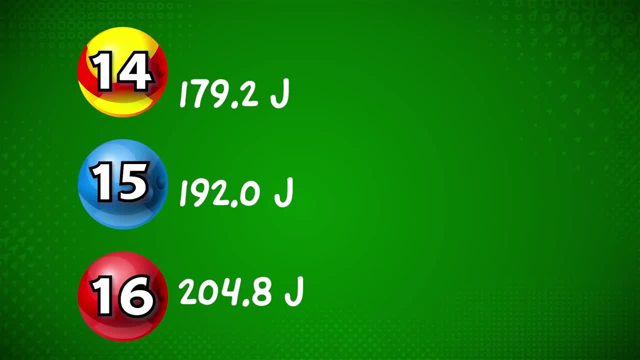 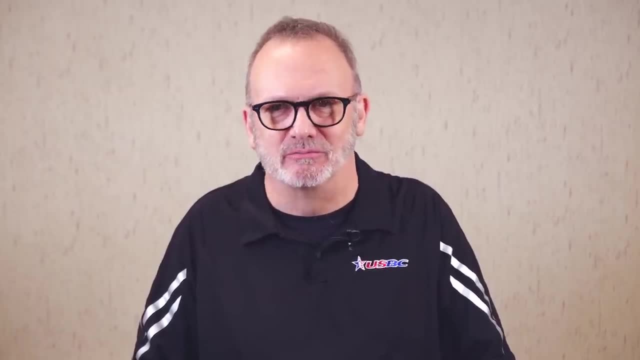 You can clearly see that the amount of kinetic energy increases for each pound added to the bowling ball. So the heaviest ball is king, right Poppycock. So let's look at this equation, Momentum being defined as the quantity of motion, of the moving 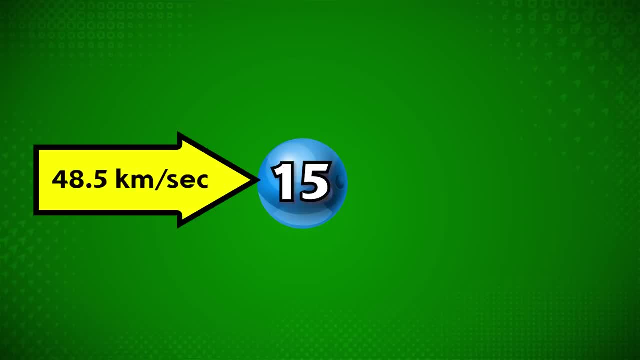 bowling ball, measured as its mass times its speed, it takes 48.5 kilometers per second of motion to throw a 15-pound ball 16 miles an hour. If we throw a 14-pound ball with that same momentum, it will travel at 17.1 miles per hour. A 16-pound ball will travel at 14.95 miles per hour.